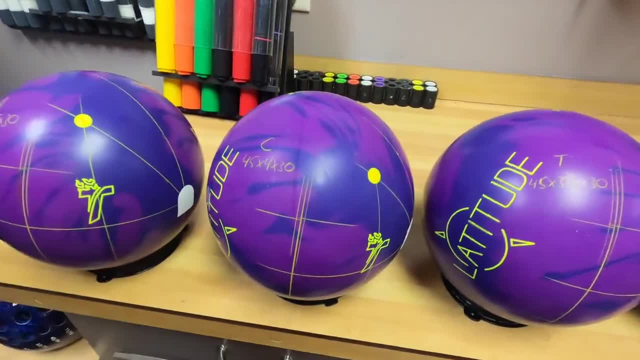 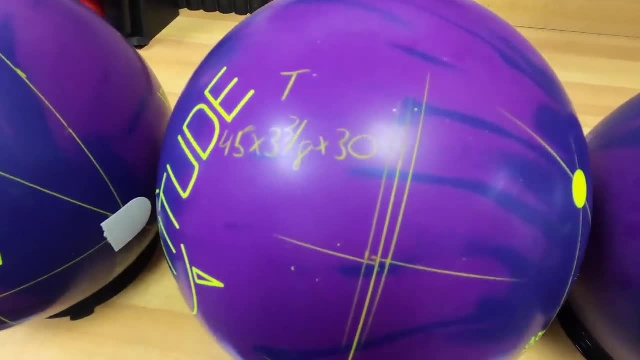 A over top of it for an angular type motion. The next ball is 45 by 4 by 30 and we put a C over top of that. for continuous motion, The third ball is 45 by 3 and 3 eighths by 30. We put a T over that. 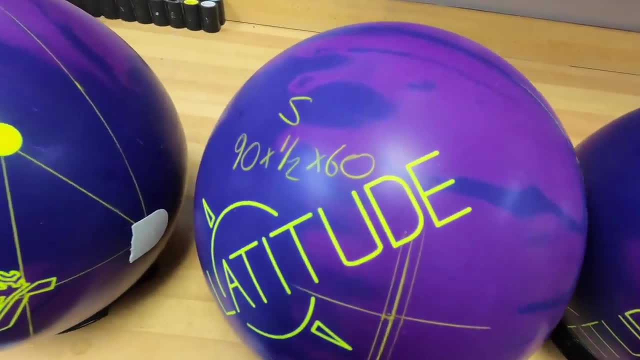 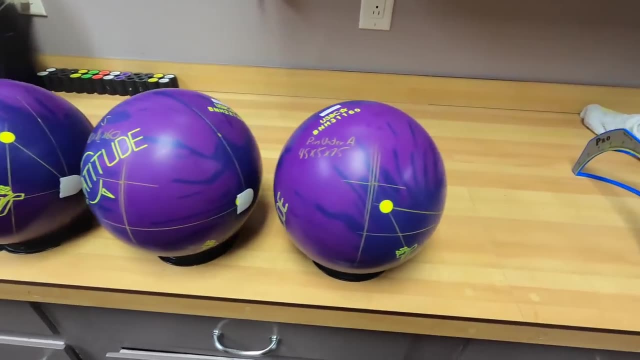 for a traction ball motion, and the fourth bowling ball we've got here is 90 by 1, half by 60, and we call this the straight ball motion. Now we've also got one other ball over here which is kind of interesting, because sometimes people like to compare pin up balls versus pin down balls. 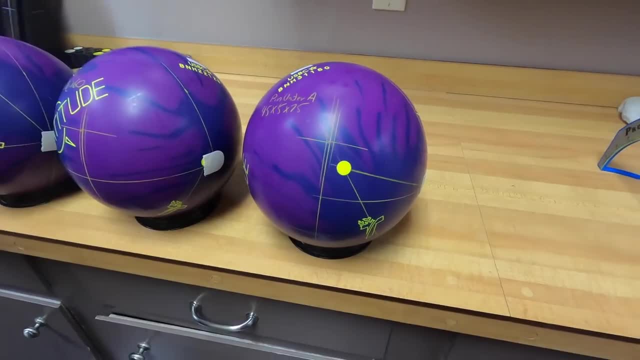 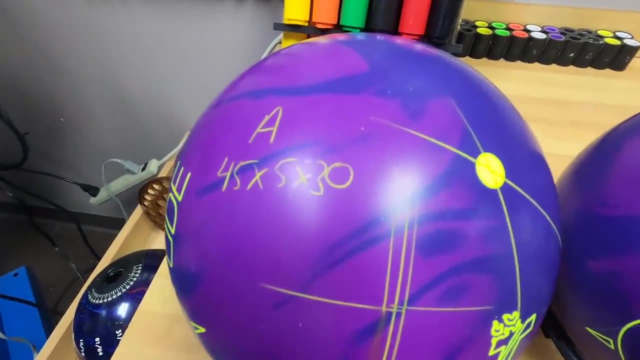 Well, this pin down ball is going to be 45 by 5 by 75. but what makes it interesting is if we go back to the other bowling ball. the other bowling ball is 45 by 5 by 30. So the only thing that's changed. 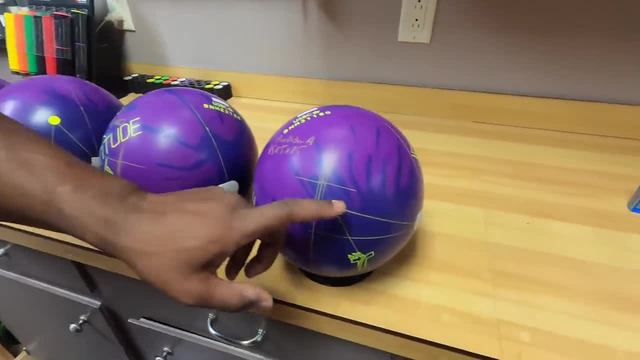 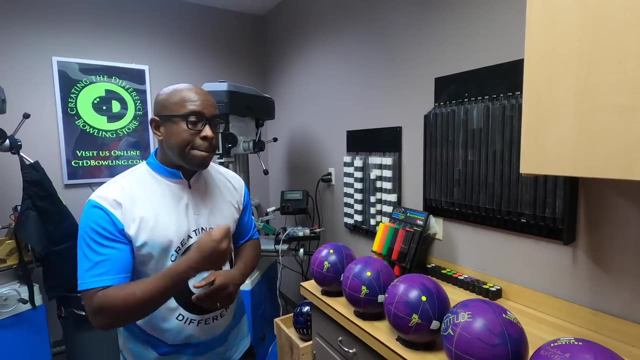 is that second angle. So the bowling balls, the pin, the PAP doesn't is the exact same, just that second angle is different. Now you may go, okay. so what are you going to do with these balls? We're going to drill these bowling balls up. We're going to throw them down a lane. We're going to get some. 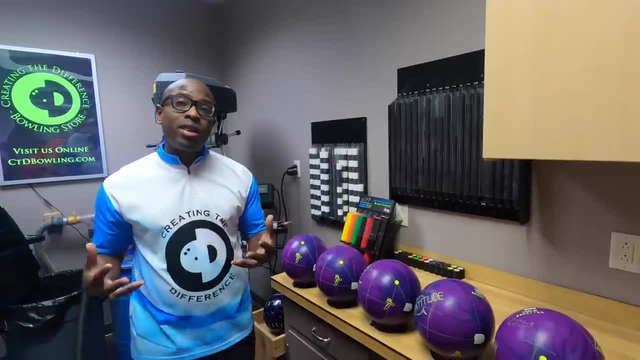 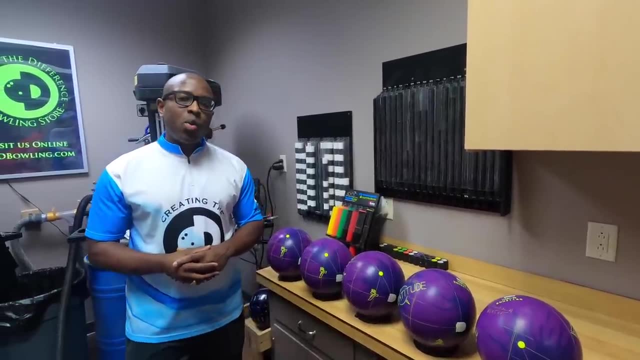 spectra data to give you some performance on what the differences are with these bowling balls. But we're going to do one other cool thing that you may find interesting at the end of the video. You'll want to stick around and watch that, because that'll kind of help answer a couple other. 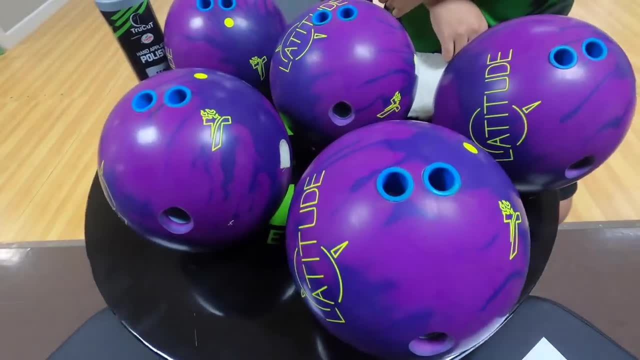 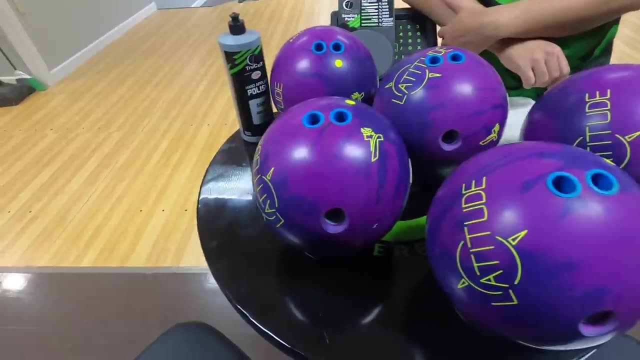 questions that you may have. Stay tuned. Today we're going to talk about layouts. It's a hot topic people always want to discuss and always want to learn more about, So we decided we would shoot a video on it. So we're going to start off by talking about five different bowling balls, but 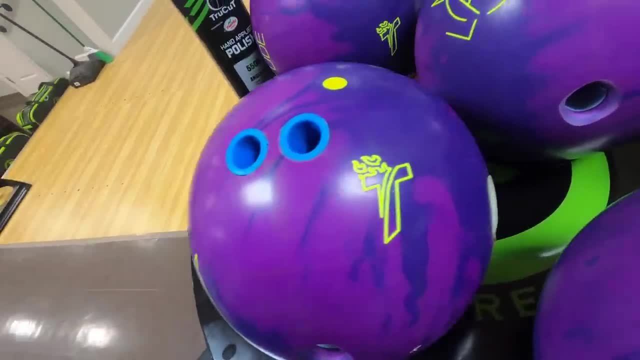 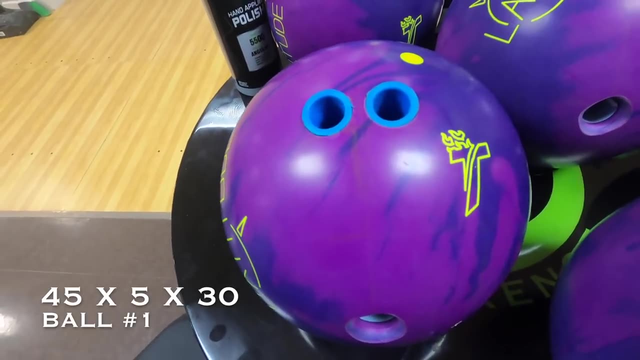 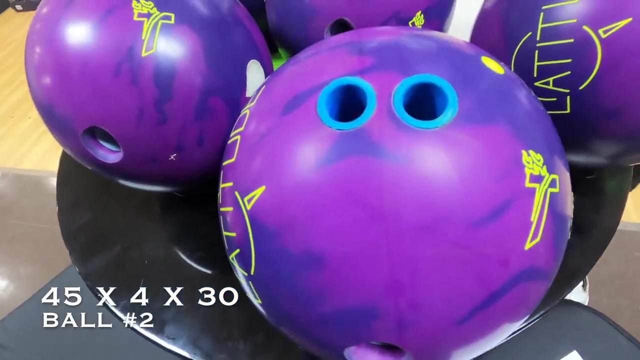 we're going to focus on four. The first ball is this one right here. We've actually marked the positive axis point with the white piece of tape on each of these balls. This ball happens to be laid out 45 by 5 by 30 degrees. This bowling ball right here happens to be laid out 45 by 4 by 30. 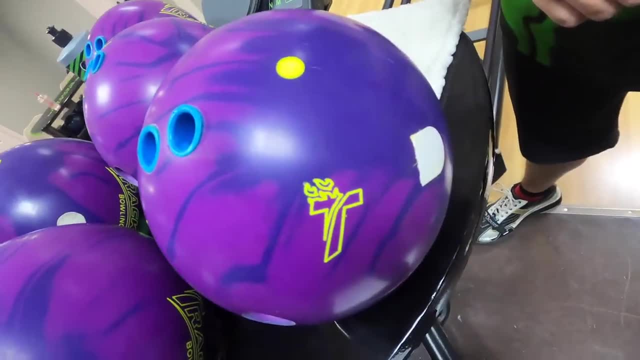 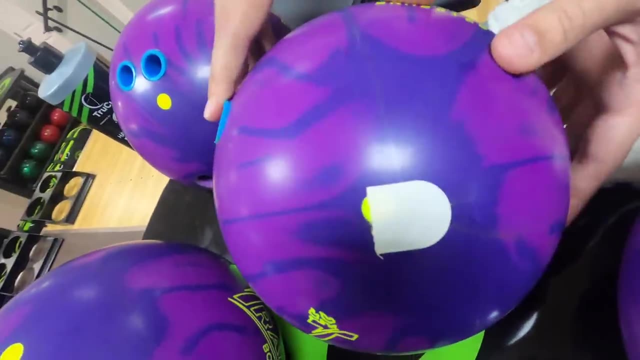 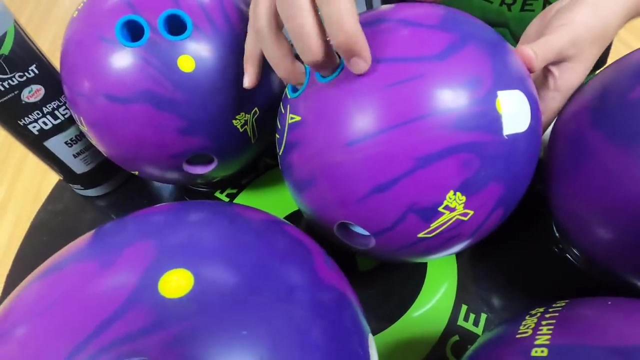 degrees. This bowling ball right here happens to be laid out 45 by 3 and 3, 8 by 30 degrees. And this bowling ball looks kind of funny, right? Look at this way. way over here, This ball happens to be laid out 90 by 1 half inch by 60 degrees. And then, last but not least, we've got one ball that's laid. 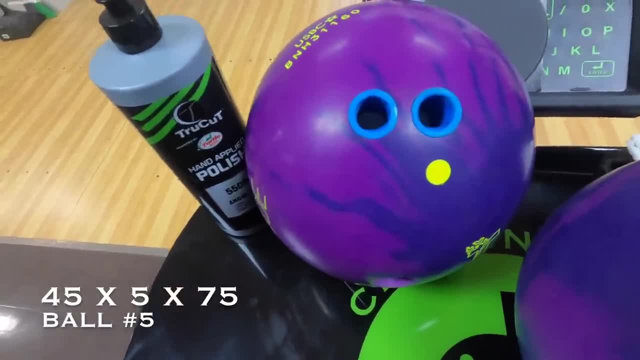 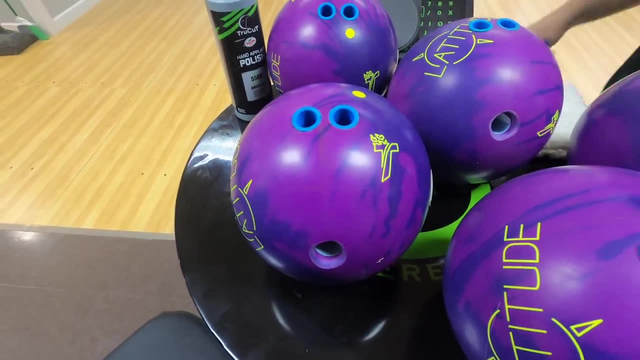 out 45 by 5 by 75, which happens to be the pin down version of this ball, which was 45 by 5 by 30. So what we're going to do is we're going to have Dustin throw some shots, So we're going to collect. 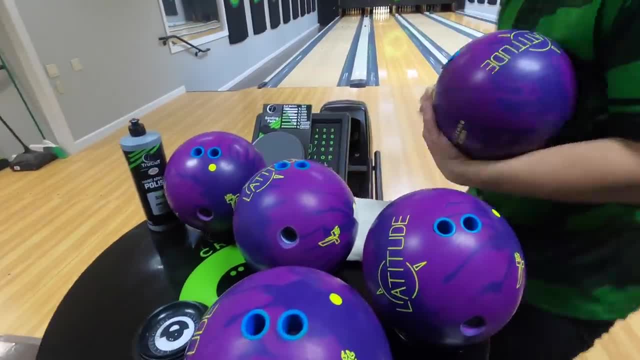 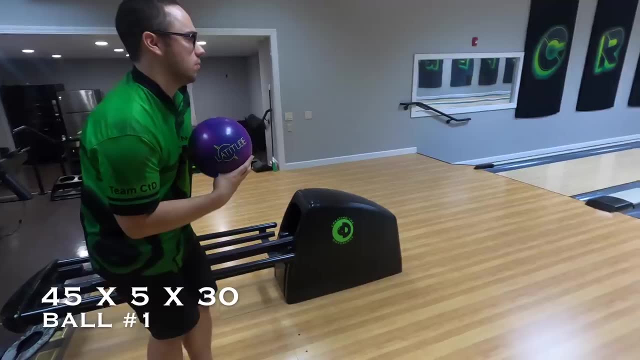 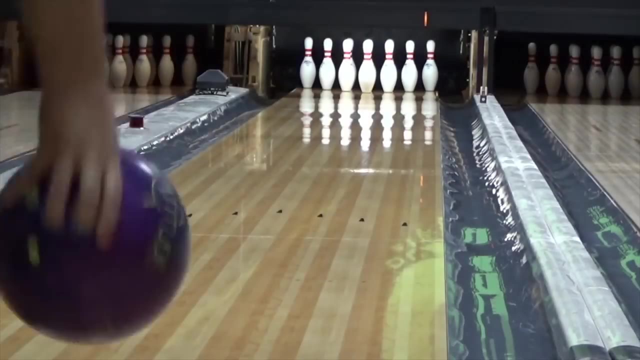 some data and we're going to talk a little bit about what we're seeing. We're going to start by throwing that 45 by 5 by 30 bowling ball, All right. so that gives us our cats, or cats, That gives us our spectro data to the peek at. So we'll take a peek at the spectro data real. 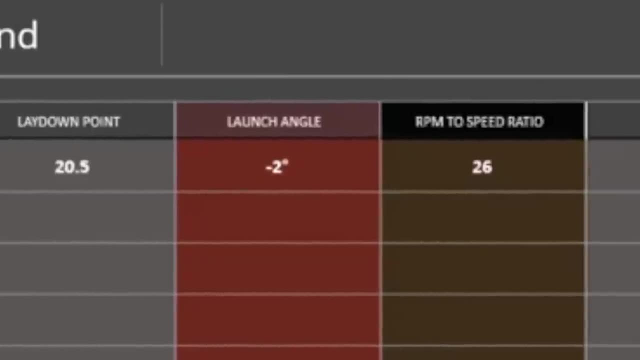 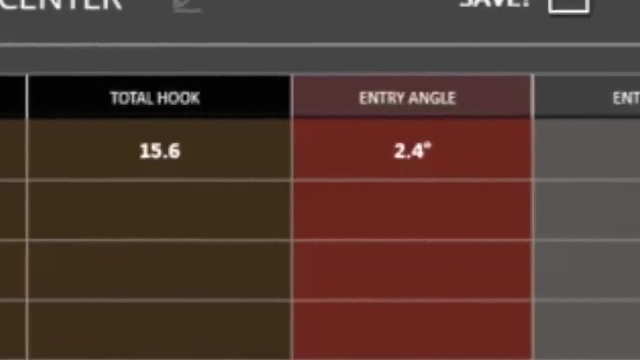 quick. The spectro data just lets us kind of see a little bit about what's going on. It doesn't really mean a whole lot at this point until we start to do some comparative testing. So we're going to put this ball up here. Take a peek at the flare pattern of that particular ball. You just 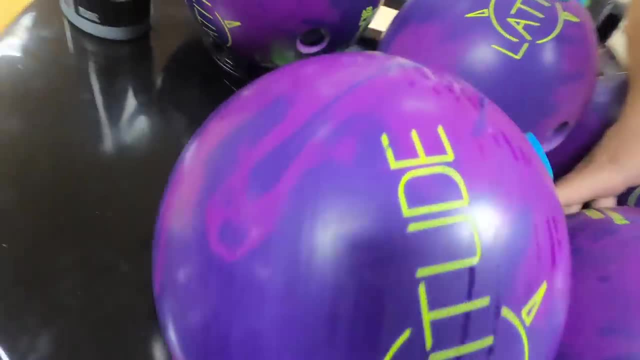 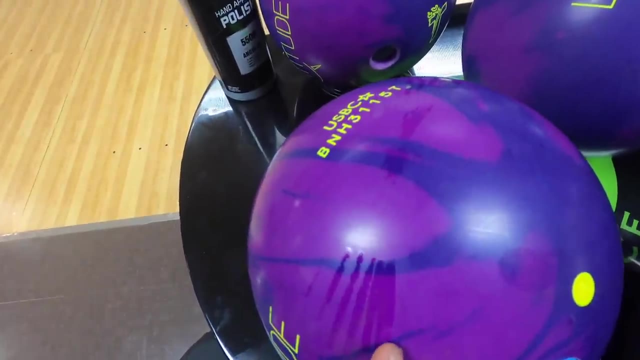 kind of see how the ball flares as it goes down the lane Back. here is some of the dry flare You can kind of see up here. this is what's called the bow tie point. So the flare is going this way on this part. 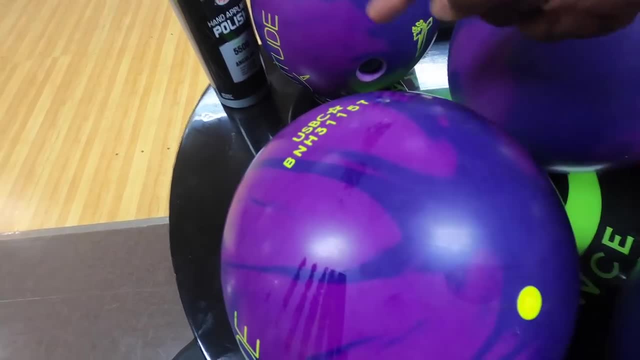 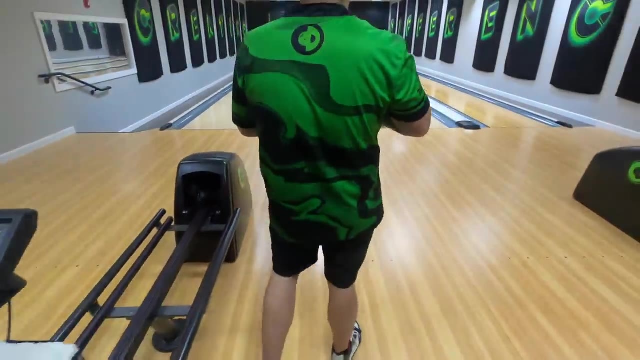 But at that, on this bow tie, it's actually going this way. So it's two different directions with the flare, and that's just kind of how the ball rolls. So now we're going to grab this ball, which happens to be 45 by 4 by 30, and we're going to show you how that ball looks as it goes down the lane. 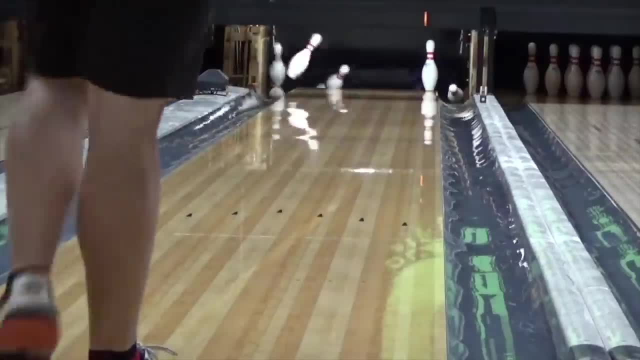 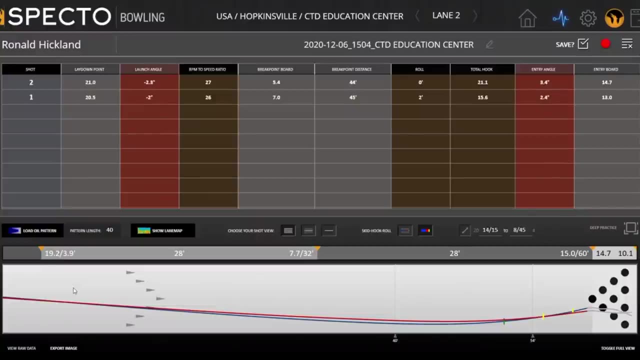 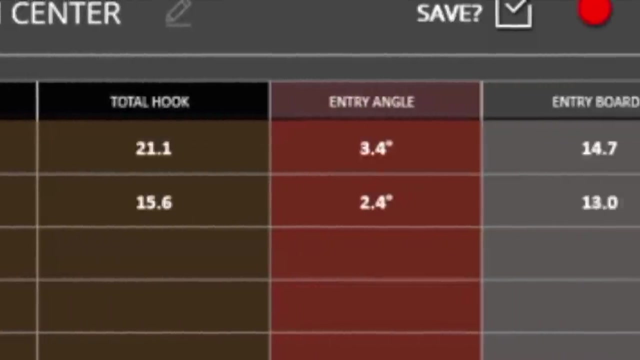 All right, We're going to throw that shot one more time: 45 by 4 by 30.. We'll delete that shot. All right, look at that shot we caught right here. Yeah, 45 by 4 by 30.. 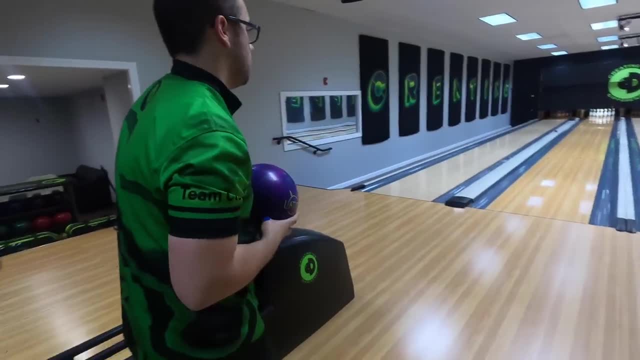 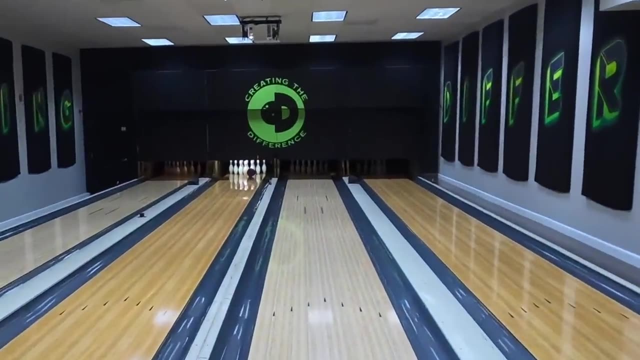 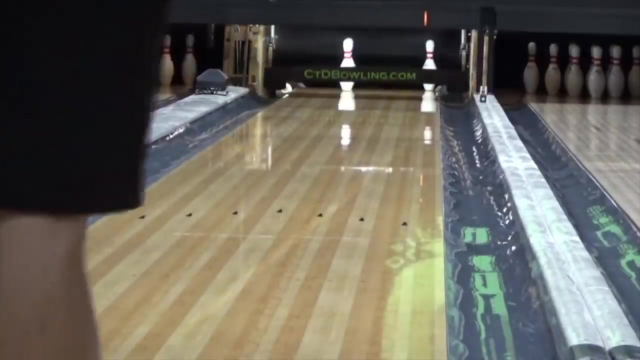 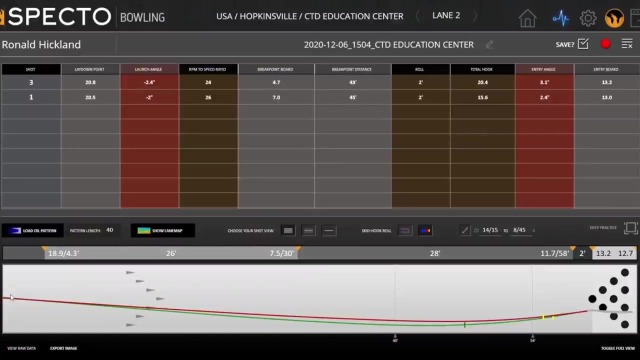 We'll throw that shot one more time. all right, looking at some of the data, launching is a little bit different there. you can kind of see that, since the launch angle is a little bit different. uh, probably have to redo that one one more time for me. 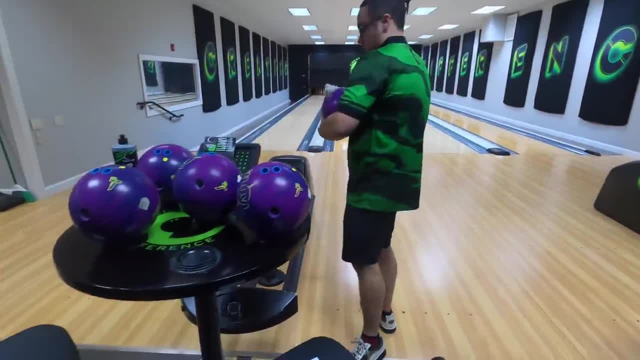 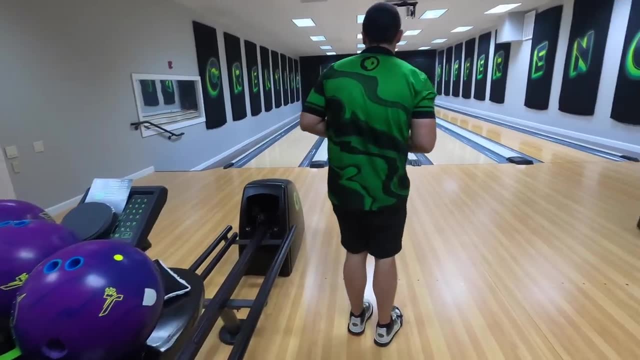 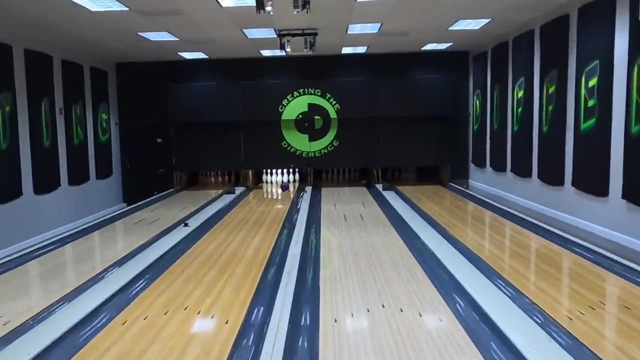 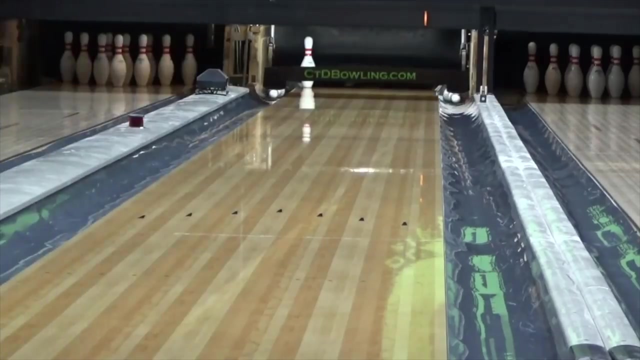 these are going to be. they're going to be very, very close, like when we get the captured shot. we're going to want to keep, we want to make sure they're really, really close. so 45 by 4 by 30.. my man's throwing wood over there, all right, that's good. so that gives us that ball. so 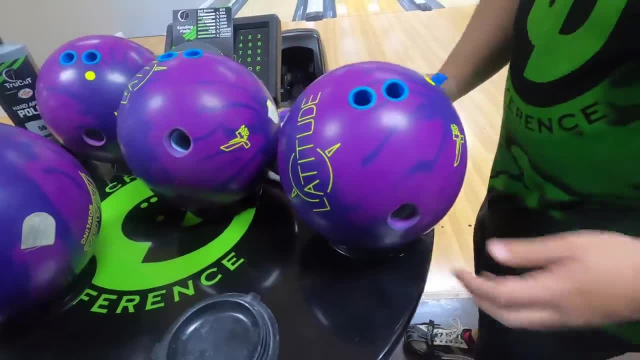 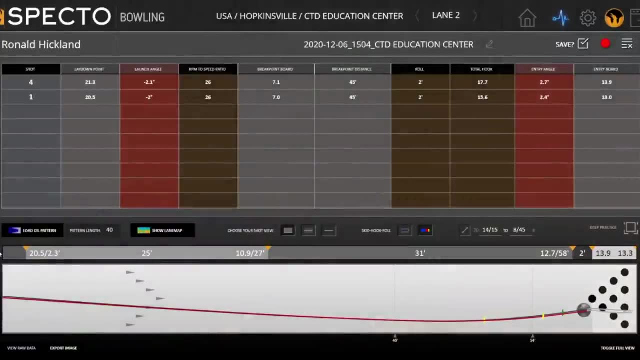 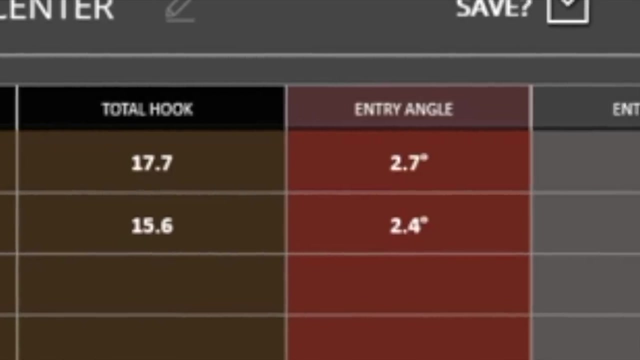 now we will move to the 45 by three and three-eighths by 30 degrees and get yourself a full rack there, and the spectro data is actually showing us just kind of how different the balls are, so you're able to see it yourself. and we're just gonna keep throwing these balls. so now we're gonna. 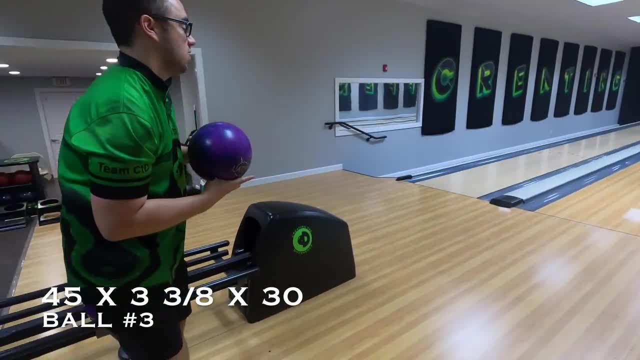 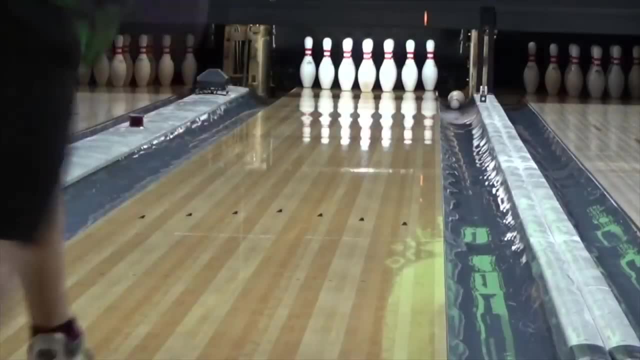 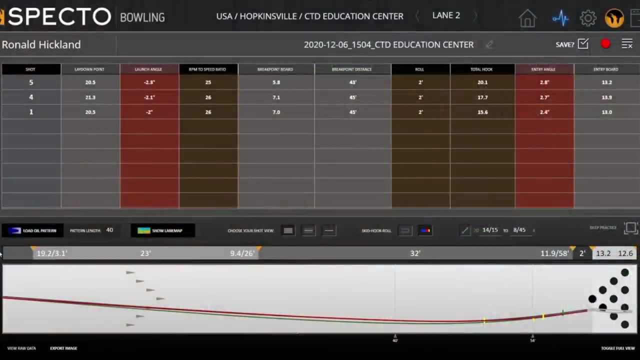 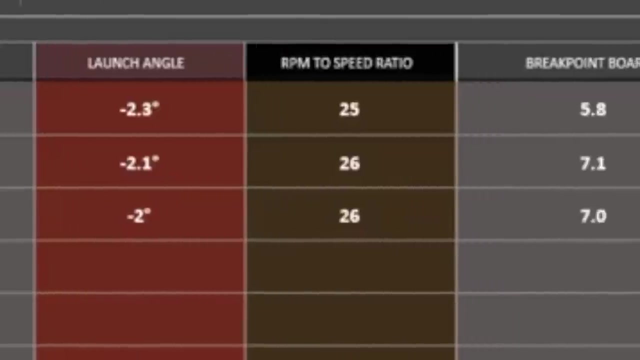 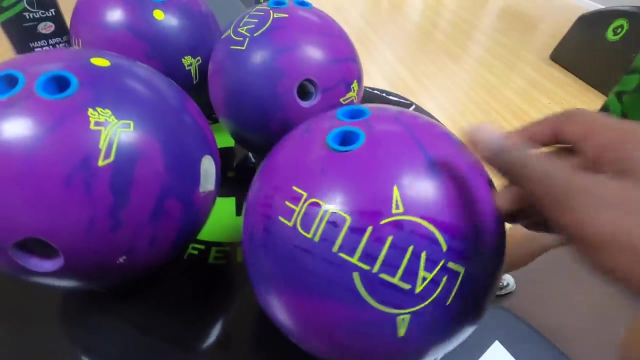 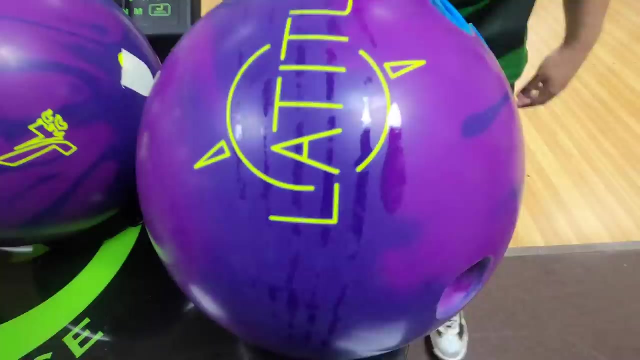 throw that 45 by three and three-eighths by 30.. all right, so we'll take a peek at that. spectra data there gives you some understanding of the future data that is go up to one in the first lap. here it goes. take a peek at the spectro data there gives you a kind of rough idea of what's going on. 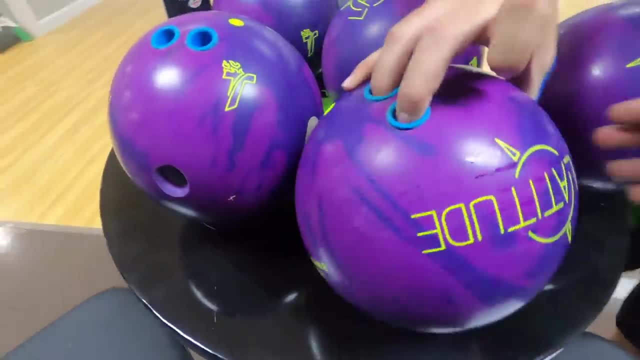 45 by 4 by 30 ball. so we'll put it up there too, just just to kind of show some of the differences. okay, so we're going to keep that shot. we're going to go to the next ball, right? so now you've kind. 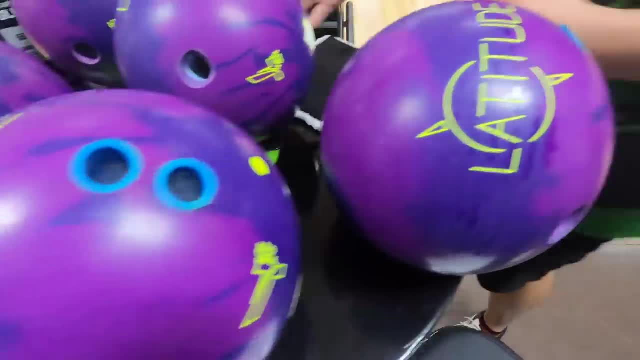 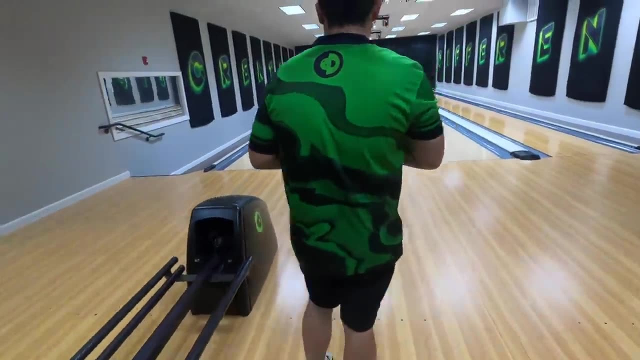 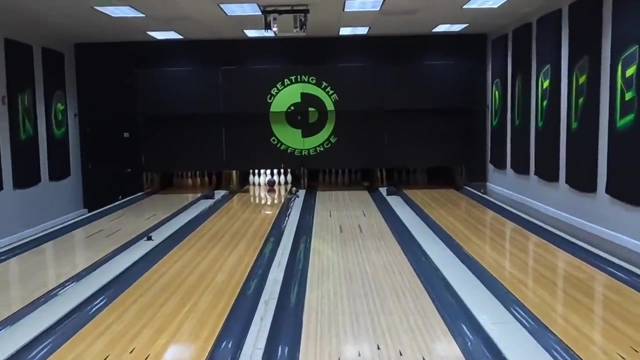 of seen three different balls, three different shots. now we're going to take a peek at this one. this is a little bit different, right? this is 90 by one half inch by 60.. all right, so now that one looks like it was in, so we're probably gonna. 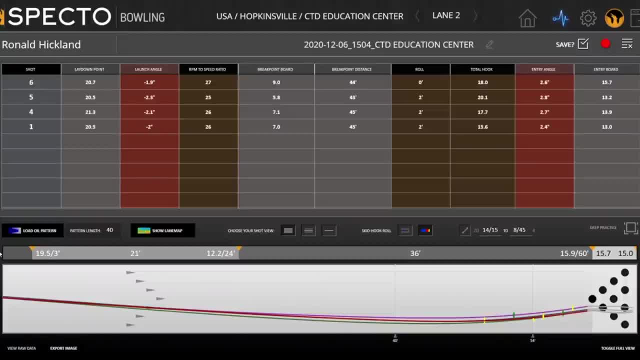 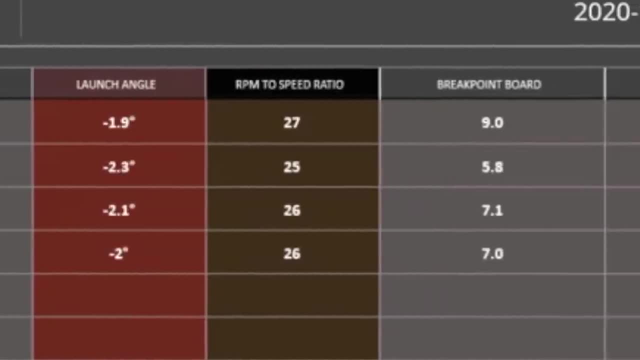 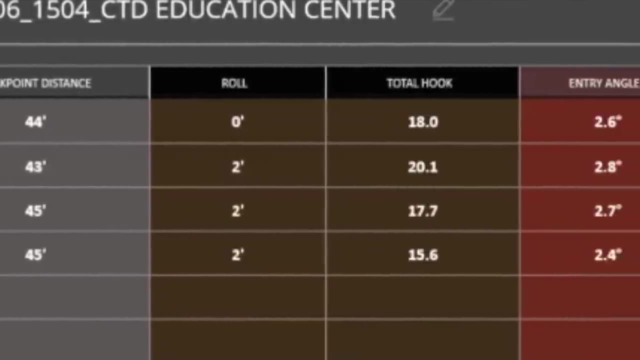 take a look at the spectro data there. yeah, is that a little bit well, but it's close, though, definitely close. let's see what those gotta say. let's have a real good look at that spectro data. actually, that one's not so bad. oh well, that's cool. so we're gonna. what we're gonna do is we're gonna keep all four of those. 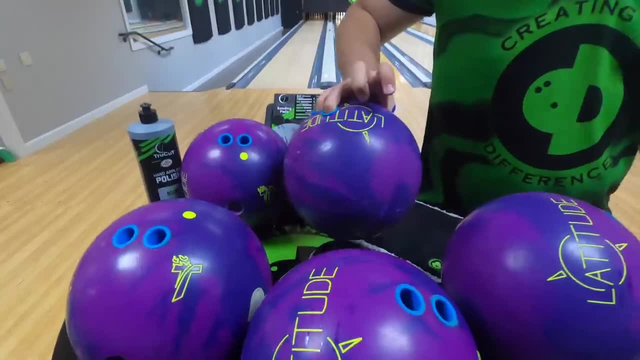 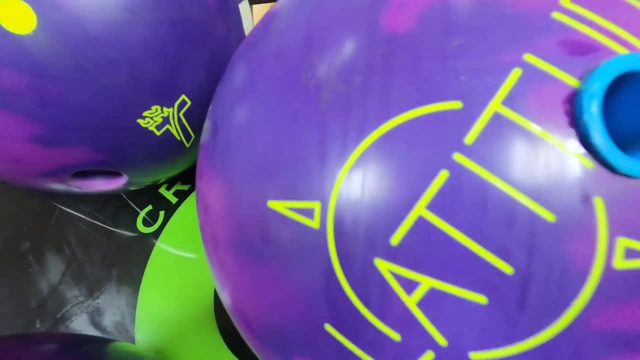 shots. um, put that ball up here. let's take a peek at it too. let's look at the flare. this is a half fish. oh, look at this. see that right there. oh, we just barely clipped that. clip that finger. that's one of the dangers of when you drill bowling balls. uh, so close to the. 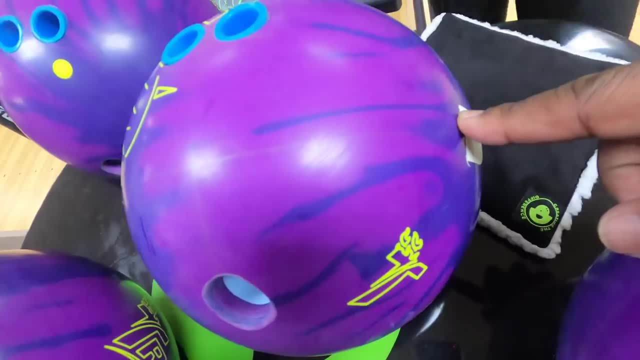 axis point and, more importantly, as you begin to bring this pin closer to the center of the grip, that bow tie point begins to move down, and that's what's causing that to actually clip. so now we're aware of that, so we're going to keep all four of those shots. um, put that ball up here, let's take a. 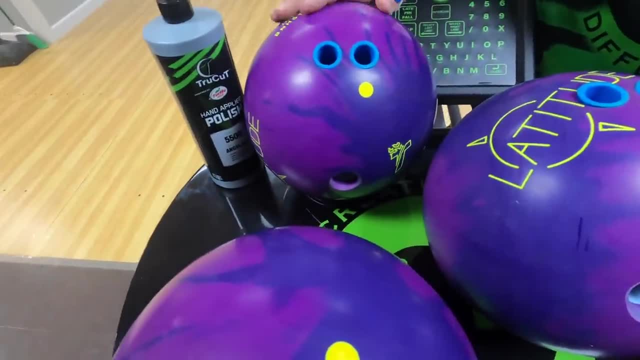 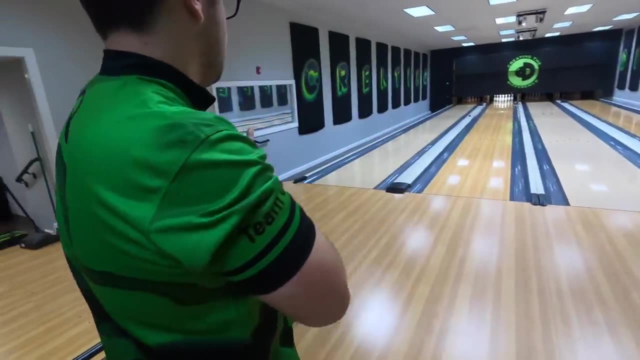 of that um as well, no big deal. we're going to throw this ball here, which happens to be 45 by 5 by 75. we're going to throw it next, and what's interesting is, you're seeing how different these balls are, or how close they are. 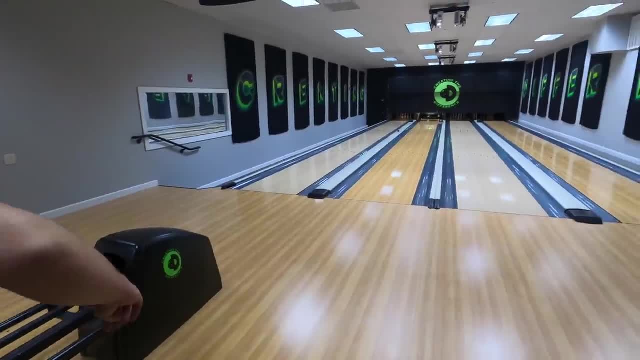 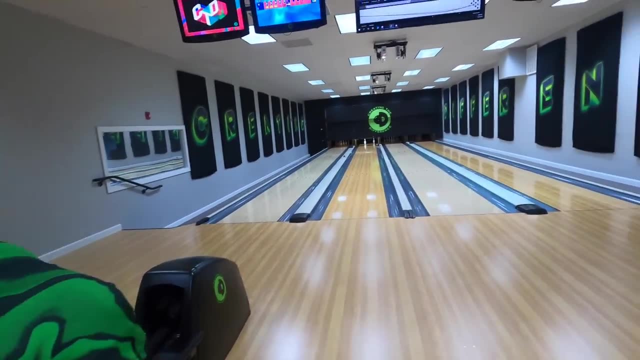 all right, so that one we will delete. we'll probably go ahead and delete that shot. launch angle was quite a bit different there, but we'll get rid of that. we'll throw it again. he'll wipe it off with that ctd bfp. keeps the bowling ball clean, gets the oil. 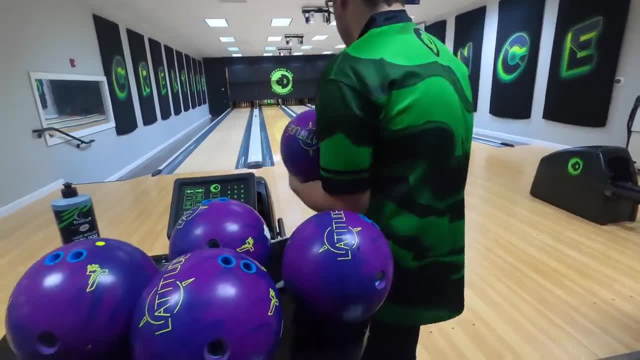 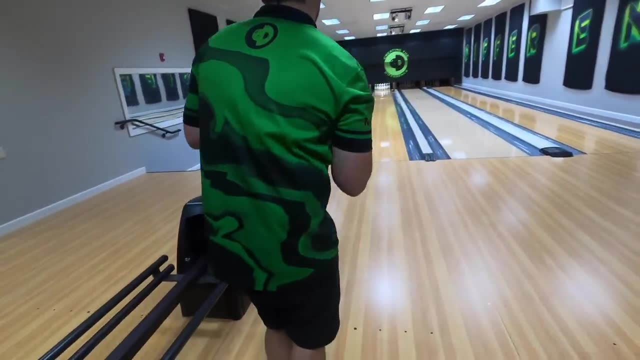 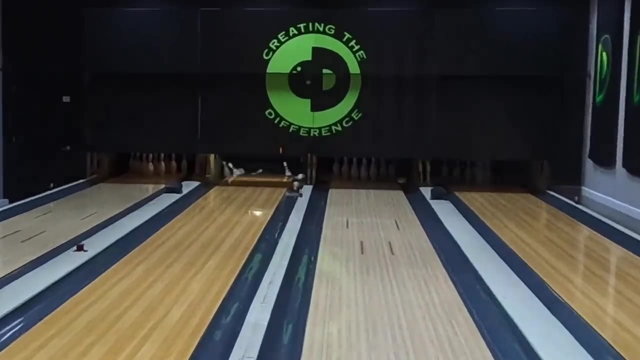 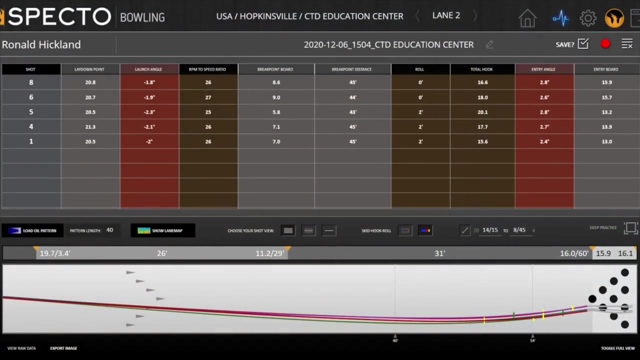 off the bowling ball, which is important, especially when you're trying to do some testing. it's important to keep that ball ball as clean as possible. so we're back on it again: 45 by 5 by 75.. oh, 10 back. the question was: did you throw it? good survey? looks like you did. looks like you did respect. 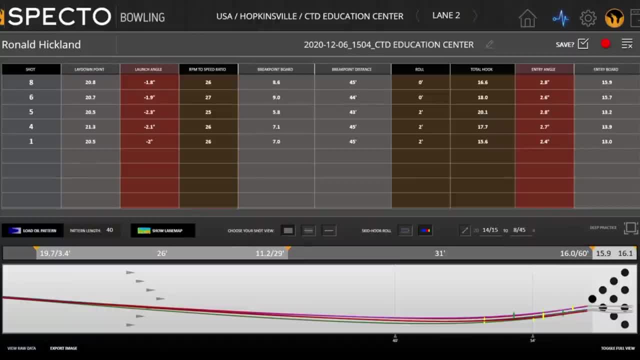 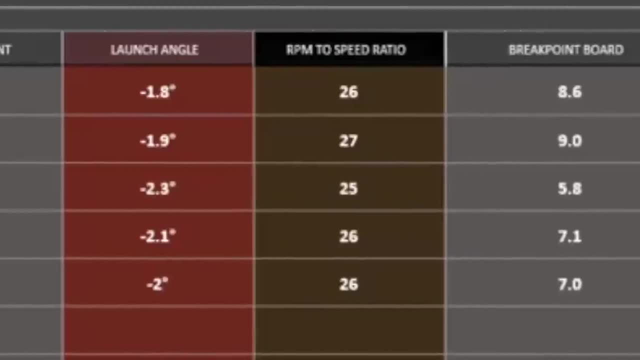 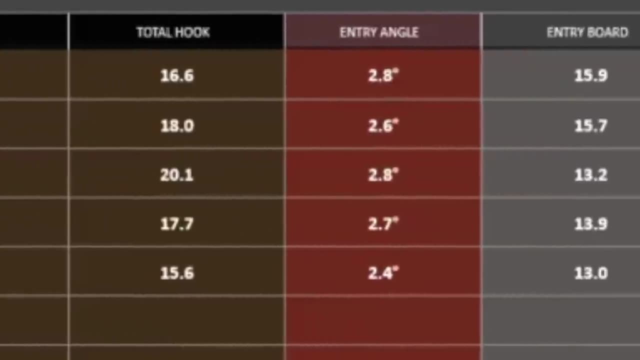 your data. i mean, look at it, look at the day, look at the day. i mean, when you're looking at this data here, you're seeing these shots are really, really close and there's a little bit of difference right. look at the total hook starting from the bottom to the top: 15.6, 17.7, 20.1, 18, even 16.6. so there's. 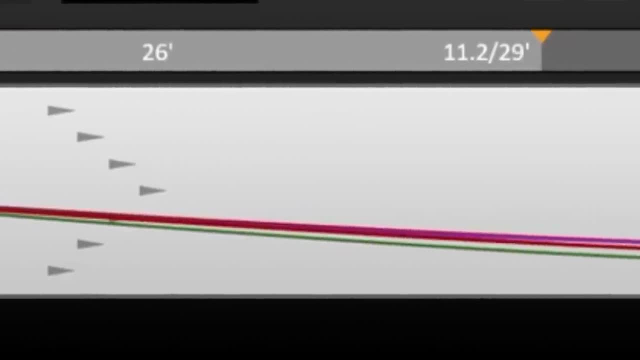 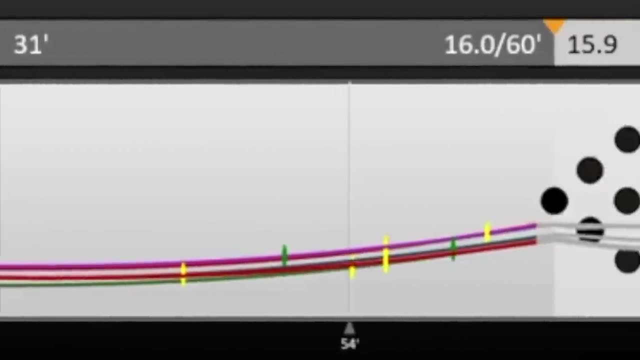 a little bit of difference there, right, and you're seeing in the data itself that you're seeing most of the change happen in the mid lane, right around 40 feet. so look at that 40 foot mark and you're going to be able to see right around. there is where there's some separation. 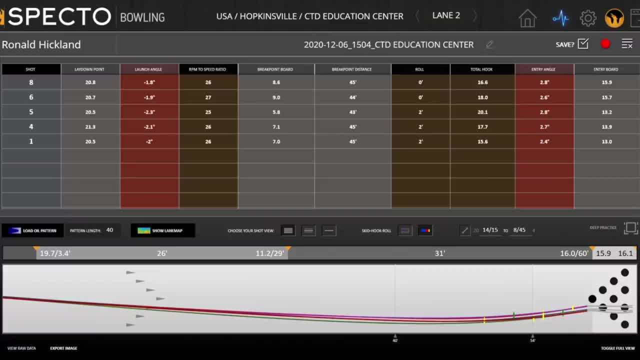 in the balls. in the back in the lane it's kind of close and the front part of the land is pretty close as well. so, ultimately, what's happening is is the data is telling you that there are some shape differences between these bowling balls kind of happens in the middle of the lane and 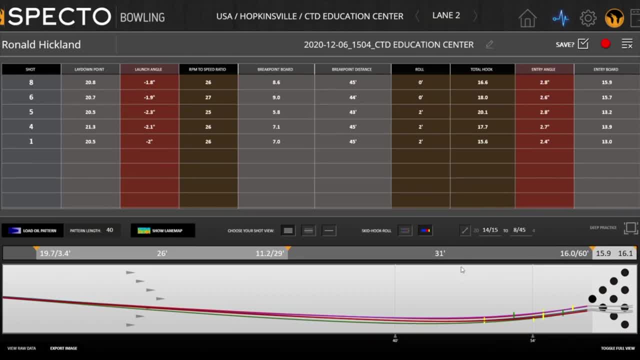 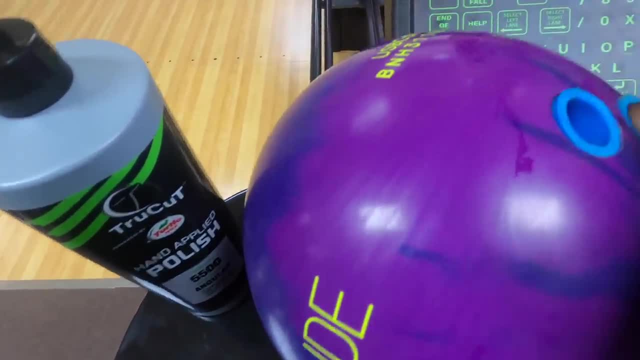 honestly, let's take a peek at the- uh, let's take a peek at the flare pattern of that ball real quick. so we're gonna look at the flare pattern of that ball too here and you can see. i mean, the flare is wide, the bow tie point is actually lower because it's. 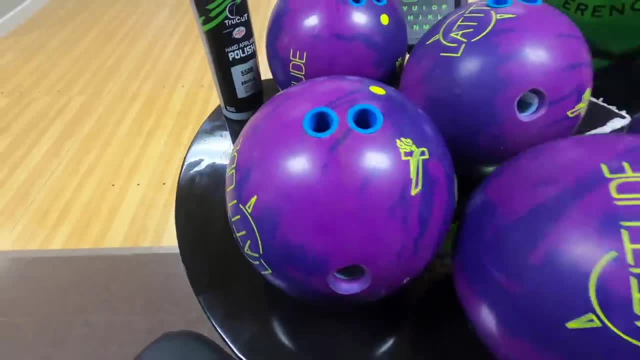 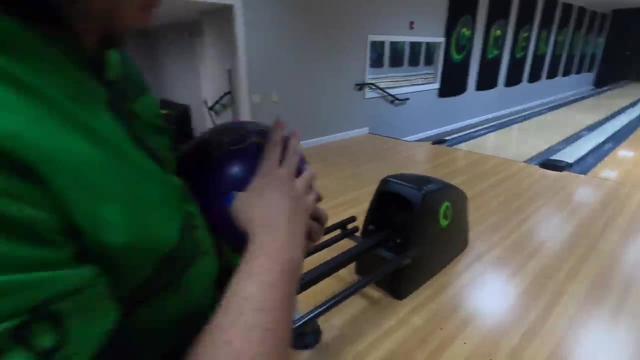 pinned down, whereas on this ball it'd actually be back here with a little pinball. pin up ball again, please. so that's, this is a really good comparison. hold on one second, i'm sorry. this is a really good comparison for you guys at home to have a better understanding of pin placement. 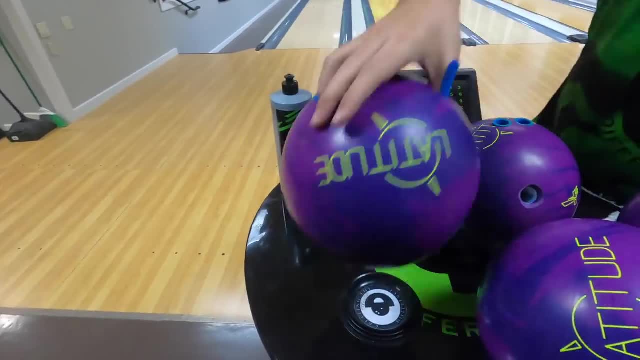 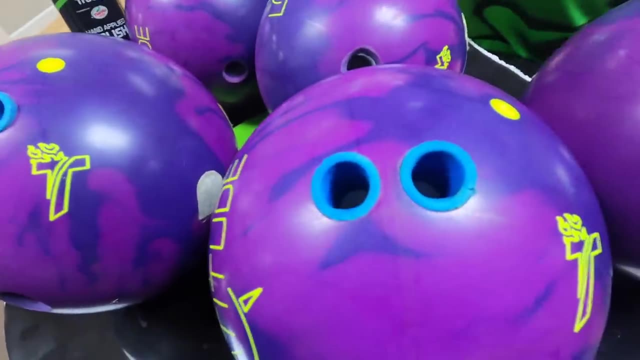 because, look, i've just shown you five different bowling balls, five completely different layouts. i mean, when you look at this bowling ball, it looks a lot different, not as too different, but a lot different than this ball right, definitely different than this one, considerably different than that one and different from that one. so they're all different. 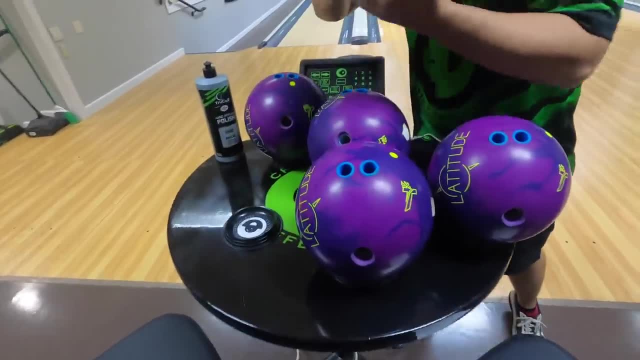 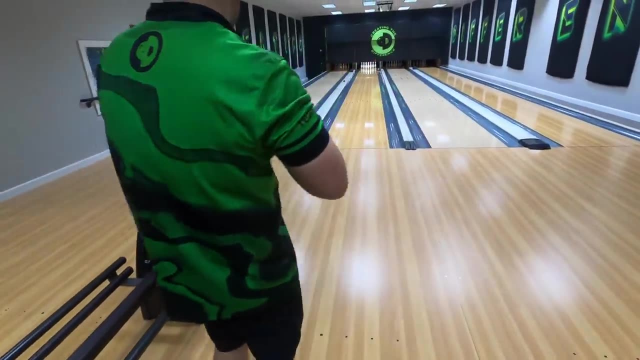 looking layouts and we're showing you the performance difference, because at the end of the day, it's the performance that matters. everybody focuses on how the pin placement looks, but really we should be focusing on how that bowling ball performs and we're seeing the most change in that. 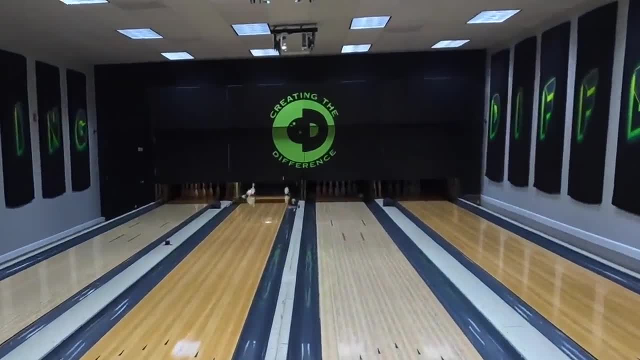 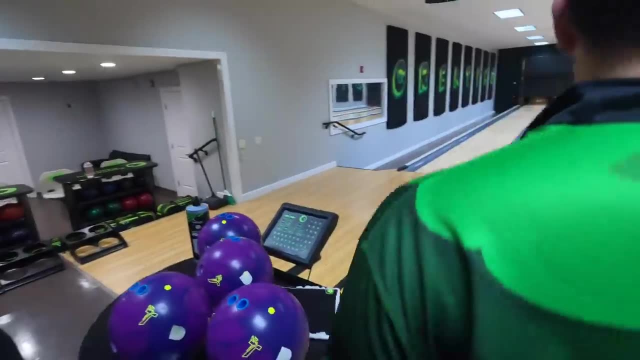 mid portion of the length. all right, fair enough, dustin. so that was the. that was the. uh, the a ball ball. um, since we will be using a 1.5 and 1.5 walk ball in the ball you want to be able to take. 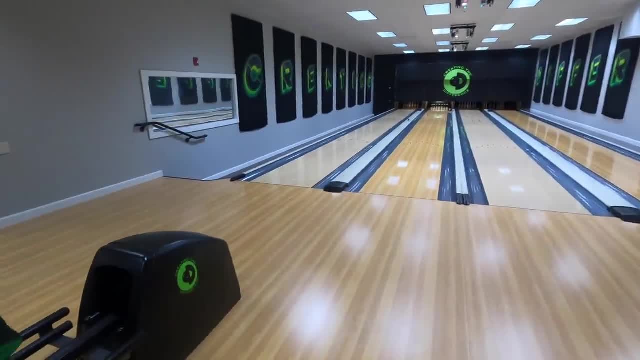 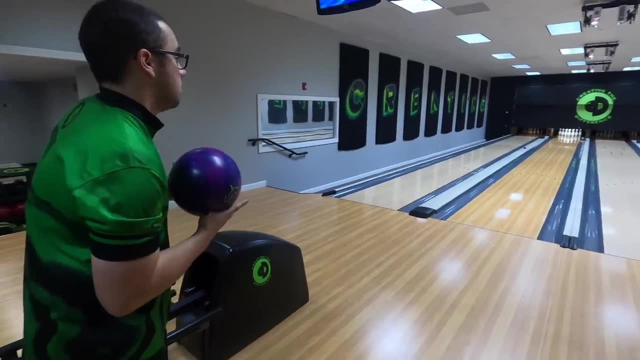 the ball out of the ball. so we know we're doing it on the ball, so we're going to do that. it's gonna be a two, three, four, five, four, six, seven, eight, eight, nine. we're gonna take a break here, right in the middle, and the ball is going to be three, five, five and a half and a half and a half. 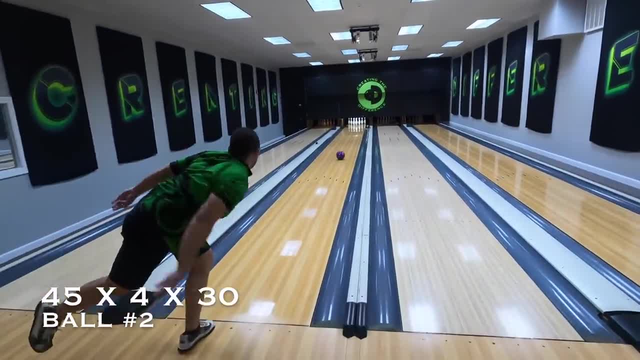 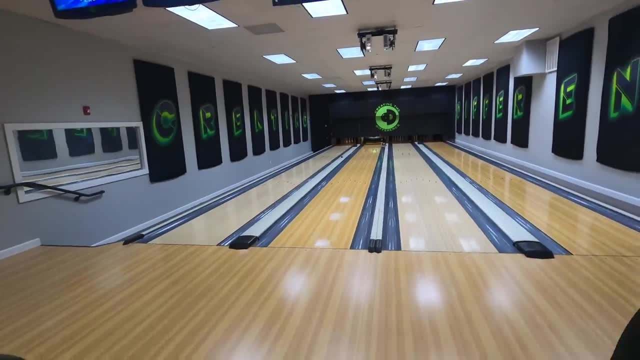 he's just a little half and a half in the middle as well, as he's gonna be doing it like a three, five or seven, five and a half and a half and a half, so you're gonna take that long ball at around seven. Next ball is going to be 45 by three and three-eighths by 30.. 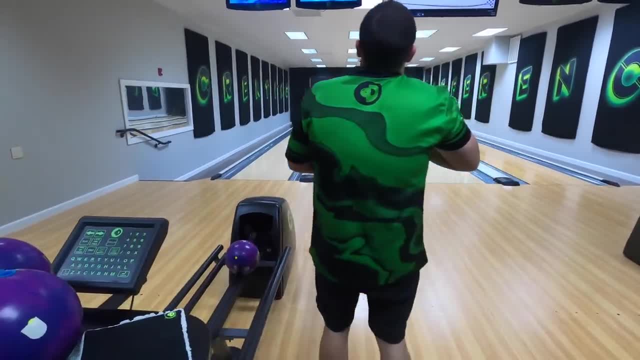 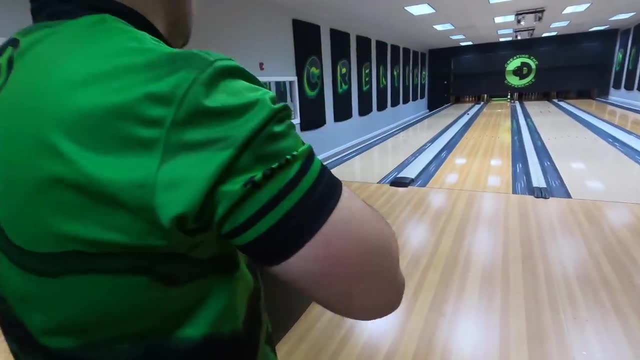 We're going to see how it rolls down the lane. So think about this, Think about what we're showing you here and the importance of this for your game. Are we seeing some differences in the balls? Yes, Is the difference massive? Not really. 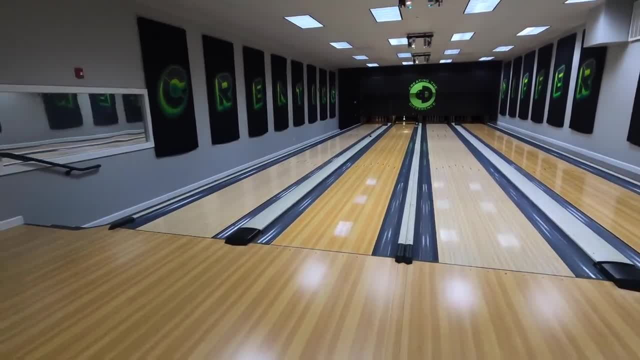 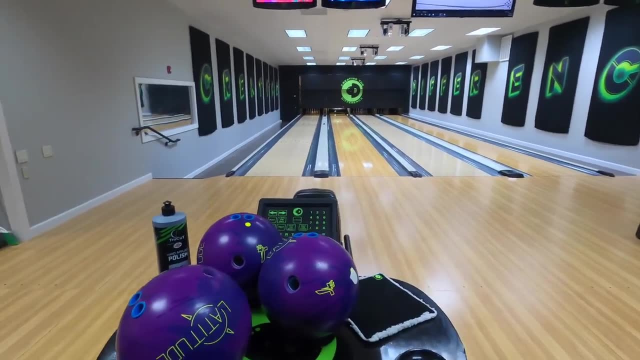 All right, Two-pin, Two-pin. We call that the traction layout. That's the one that's supposed to kind of be a little bit rollier a little bit earlier, and you can kind of see that obviously, because of that it didn't get back. 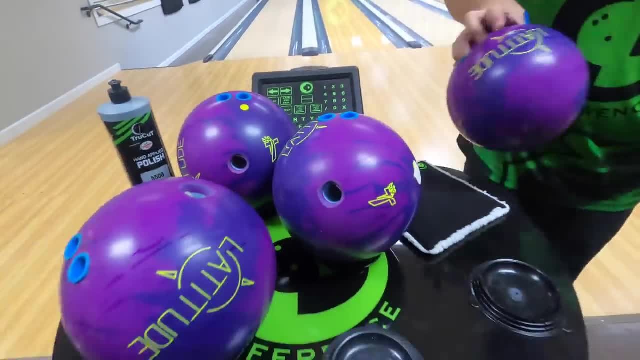 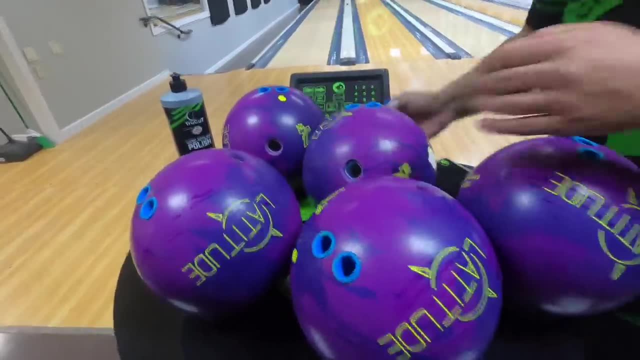 So now we're going to grab that half-inch pin layout, right, This is the one that we call the straight layout, so to speak, because the pin is a half an inch away from the positive axis point, which is going to really minimize that flare potential. 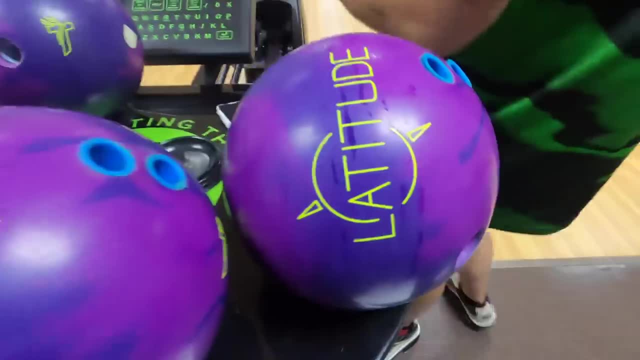 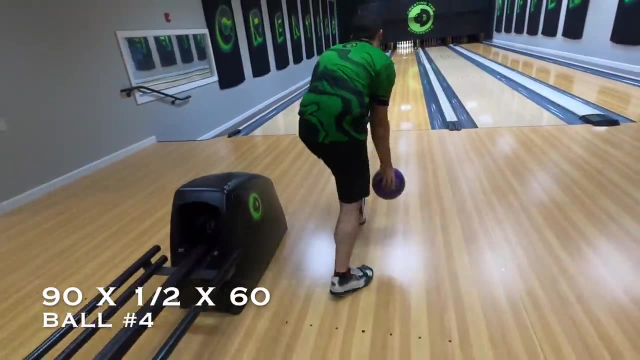 And you can kind of see the flare patterns on these bowling balls too. You can kind of see that on the bowling balls Some differences, Some differences there too. So 90 by 60 by 90, by a half, by 60.. 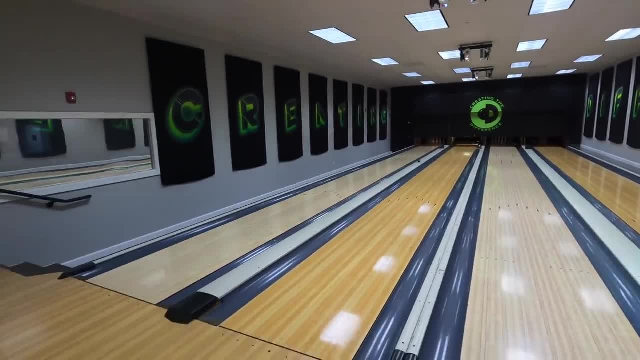 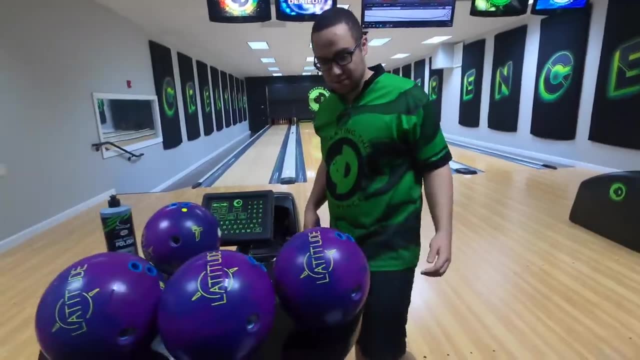 And he's going to get it. Of course, Of course, Of course. There we go, Atta boy. So I mean, you're seeing he's able to strike with all the balls. He's not moving, He's trying to repeat the exact same shot. stay in the same part of the lane. 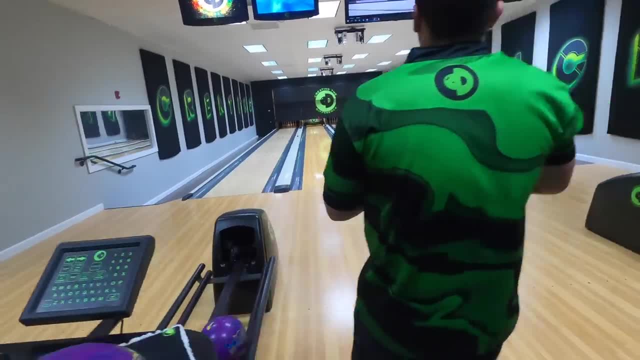 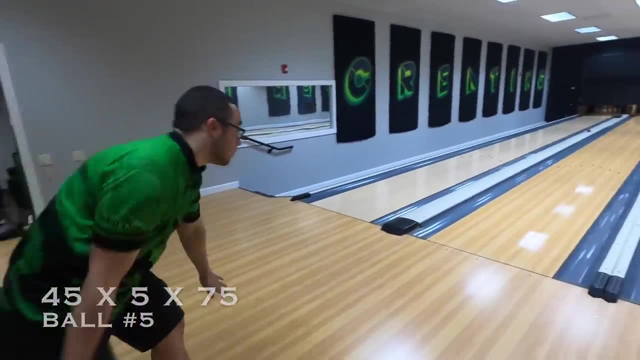 He's going to throw the pin down ball which is 45 by 5, by 75 next. And I just want you to watch, because that's really the key here, right? It's just a good understanding of what's actually happening from a ball motion. 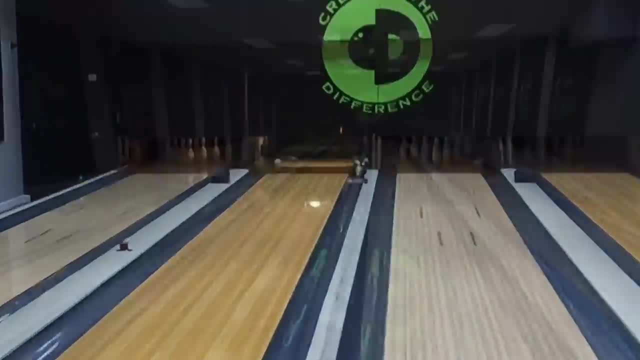 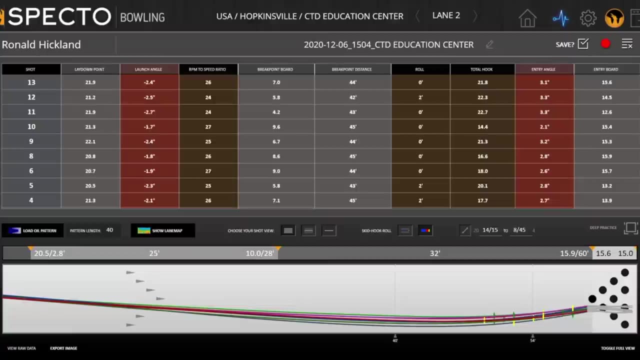 standpoint and how much difference there really is with the pin And then another strike, So Dustin's throwing all those bowling balls. The data is super, super tight. We're going to take a peek at the Spectral data right now. You can see that the data shows that we're pretty close all the way around with those bowling balls. 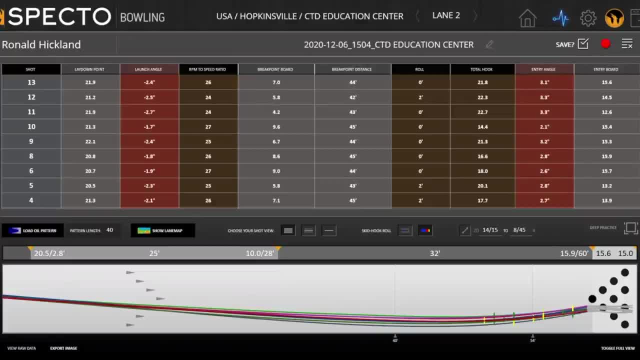 And especially, you know when you really look at the data. if you take a deep dive into it, it kind of gives you some information. there We got one shot that looks kind of funny right there at number 10.. That number 10 shot definitely looks a little bit funky. 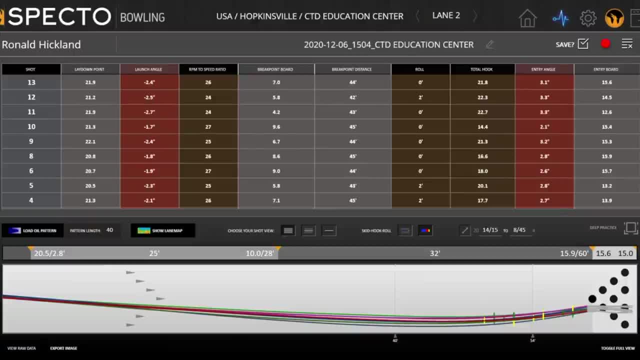 Maybe we had a little. We're going to take a look up there with the data. No worries, No worries. At the end of the day, the point we're trying to make here is you're being able to watch the ball go down the lane. 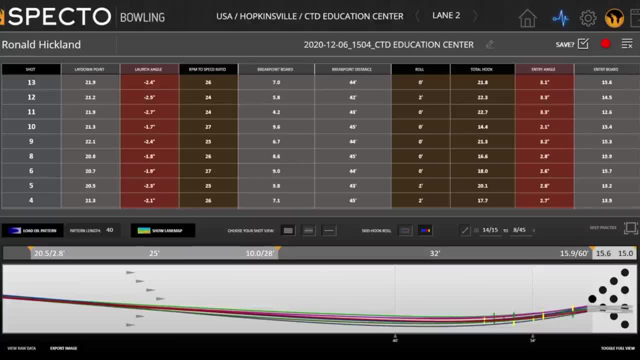 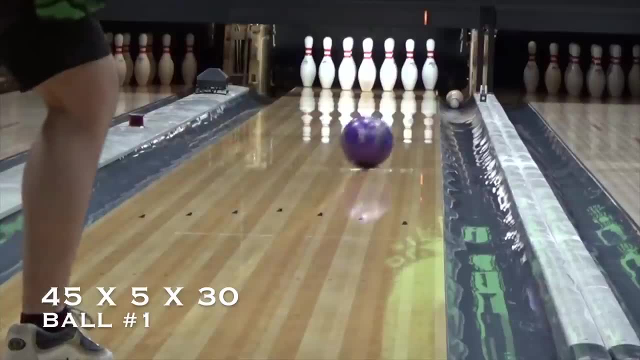 You're being able to see it yourself And, as a result of that, you're seeing just really how much difference there is or isn't when it comes to bowling ball layups, And, depending on your skill level, depending on your average level, this is going to be probably not a whole lot more different. 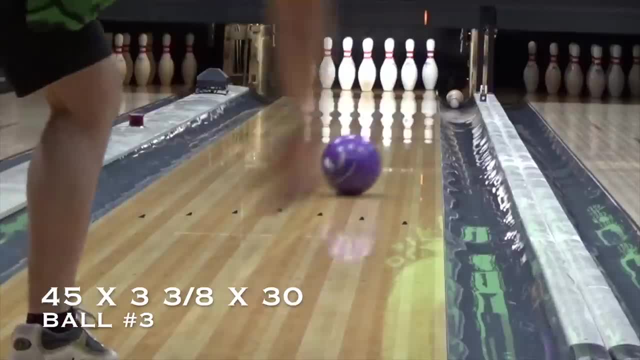 Right, But it definitely could be a whole lot less different. Dustin's a high caliber, 230 plus average former junior team USA player who repeats shots. Dustin's a high caliber, 230 plus average former junior team USA player who repeats shots. Dustin's a high caliber- 230 plus average former junior team USA player who repeats shots. 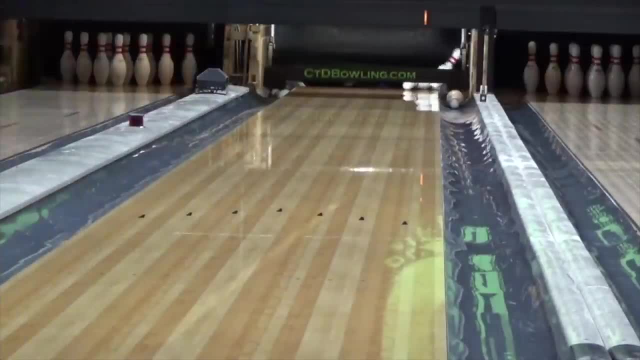 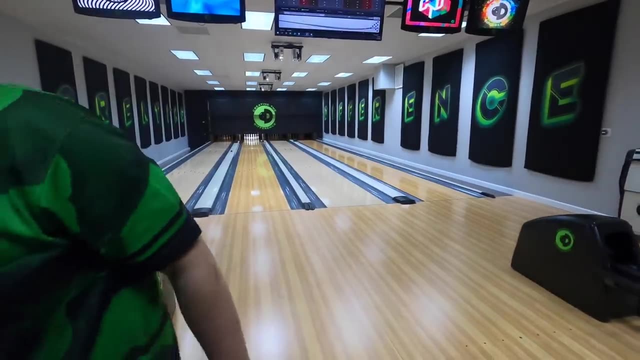 Imagine what happens if you are a 180 average bowler or a 200 average bowler who doesn't repeat shots, and you've got all these different layouts. What's going to end up happening is you're going to end up seeing a lot of your bowling balls do the exact same thing because, quite honestly, we're showing you what the difference is when you do repeat the shots. 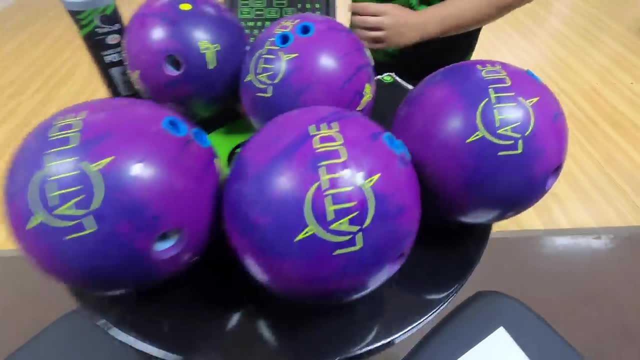 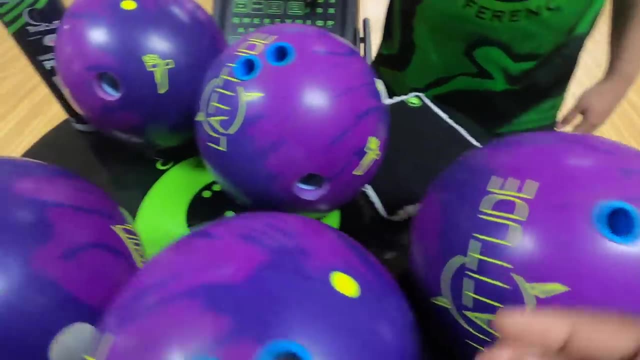 So now you got a little bit more information. You've got some more insight onto the power of layouts, And maybe there's a layout that you like that's better for your game. You also learn a little fact, too, about putting the ball pin under right.